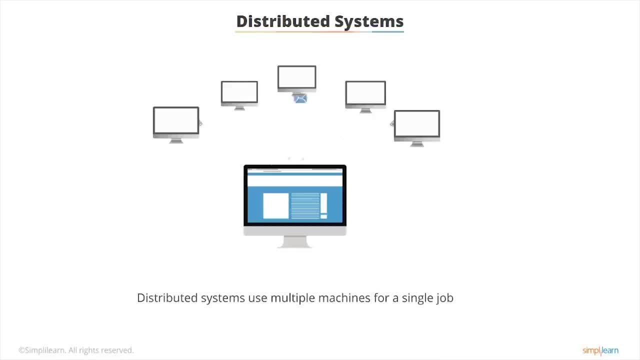 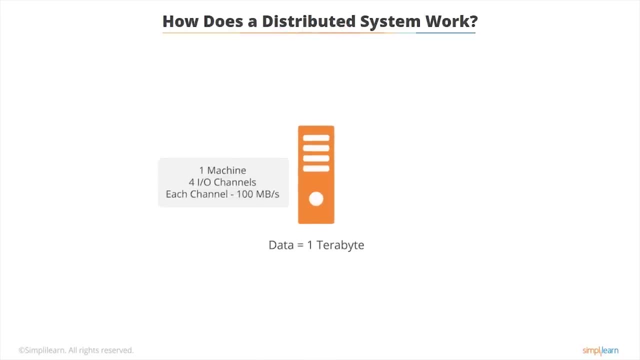 multiple machines. This is called distributed system. Let's look at an example to understand how a distributed system works. Suppose you have one machine which has four input-output channels. The speed of each channel is 100 megabytes a second And you want to process 1 terabyte of data on it. How much? 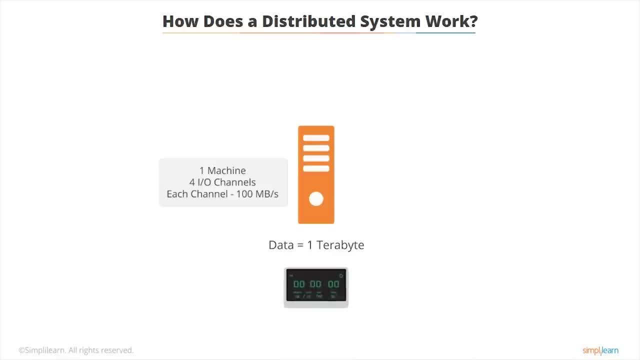 time do you think it will take to process the data? It will take 45 minutes for one machine to process 1 terabyte of data. Now let's assume 1 terabyte of data is processed by 100 machines with the same configuration. How much time do you think it will now take? 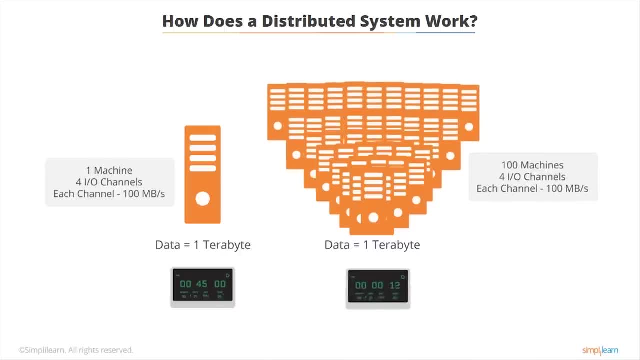 to process the data. It will take only 45 seconds for 100 machines to process 1 terabyte of data. Distributed systems take less time to process big data. Now let's look at the challenges of a distributed system, Since multiple computers are used. 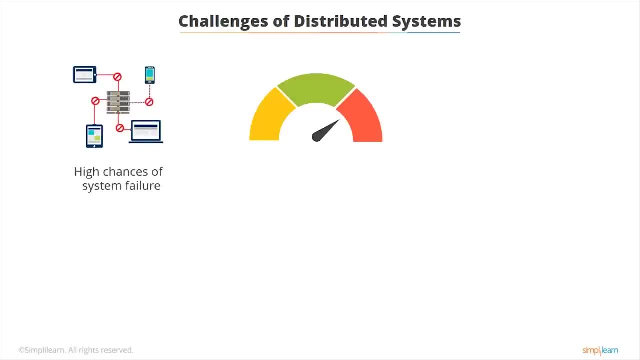 in a distributed system, there are high chances of system failure. There is also a limit on the bandwidth. Programming complexity is also high because it is difficult to synchronize data and process. Did you know the solution to these challenges? Hadoop. So what is Hadoop? 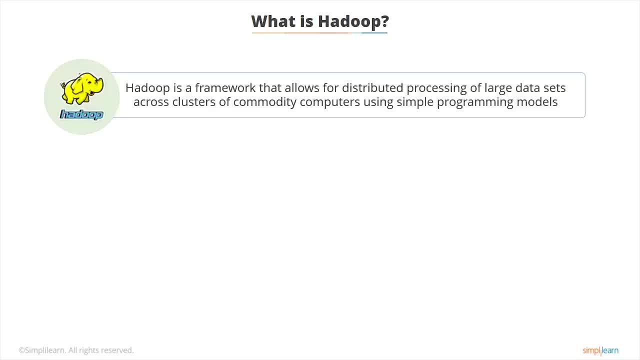 Hadoop is a framework that allows for the distributed processing of large datasets across clusters of commodity computers using simple programming models. It is inspired by a technical document published by Google. The word Hadoop does not have any meaning. Doug Cutting, who discovered Hadoop, named 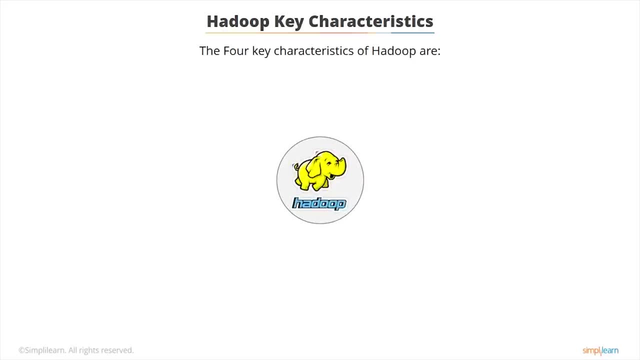 it after his son's yellow-colored toy elephant. Let's discuss how Hadoop resolves the three challenges of the distributed system. How does Hadoop solve the three challenges of the distributed system? How does Hadoop solve the three challenges of the distributed system? 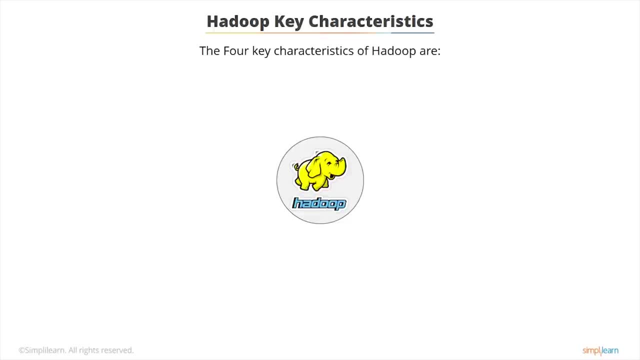 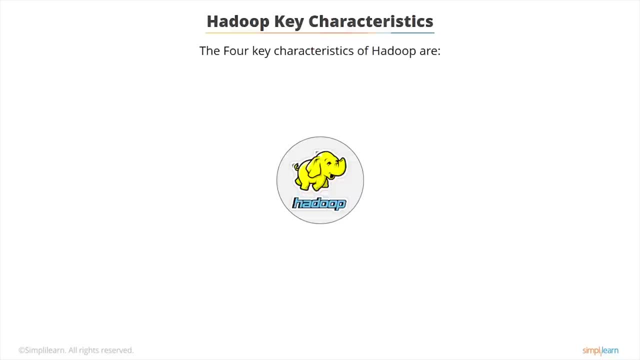 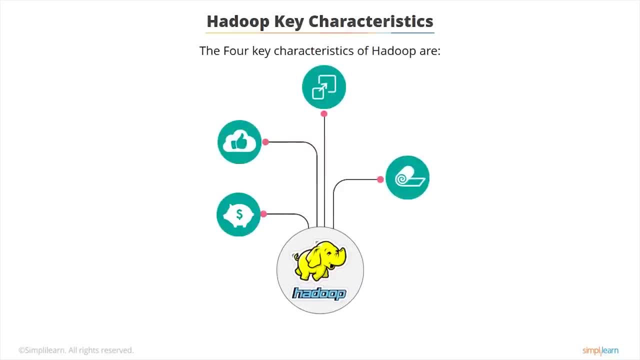 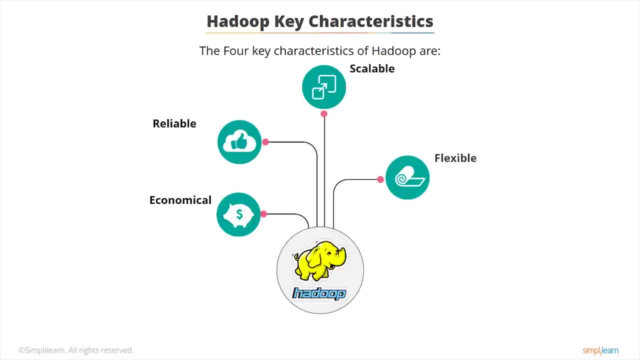 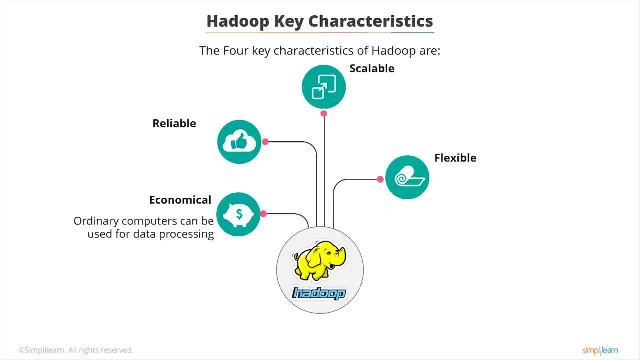 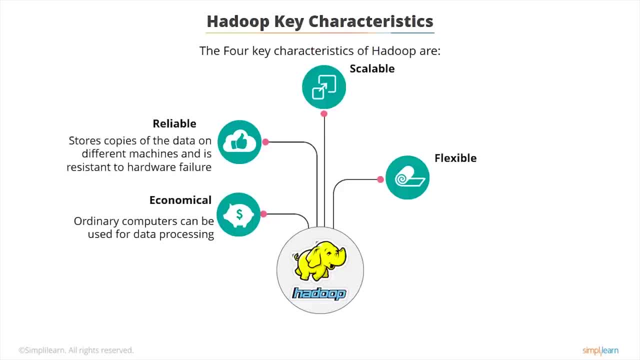 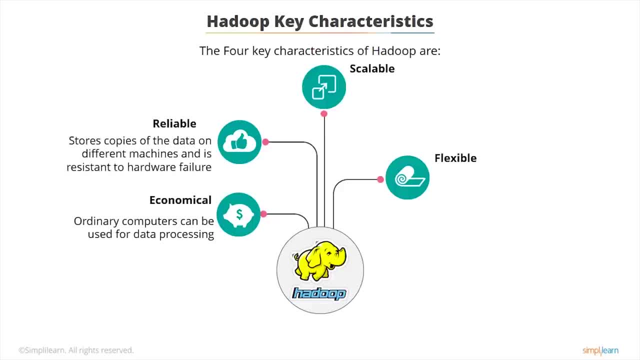 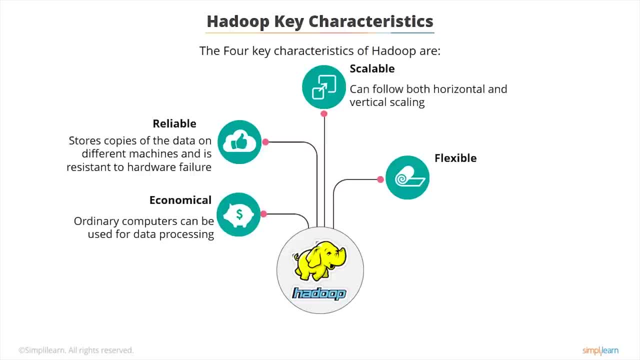 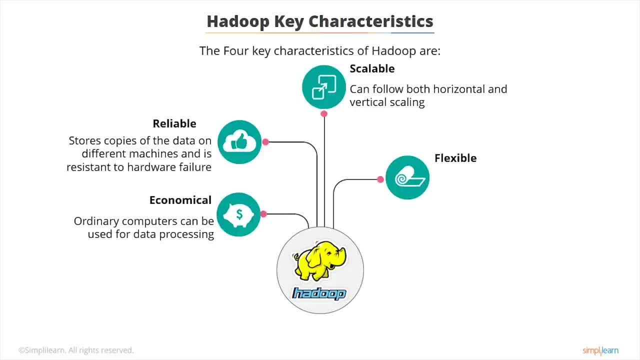 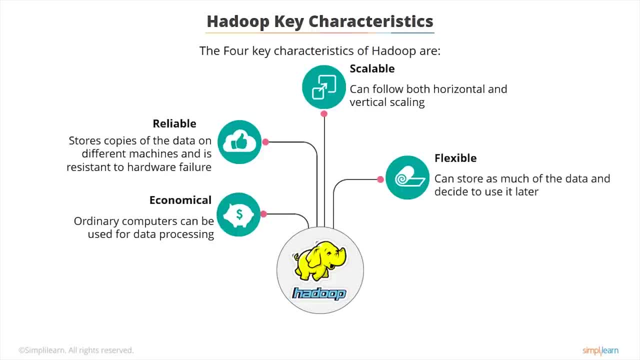 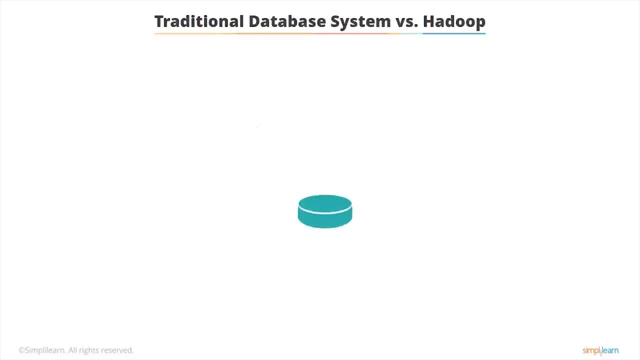 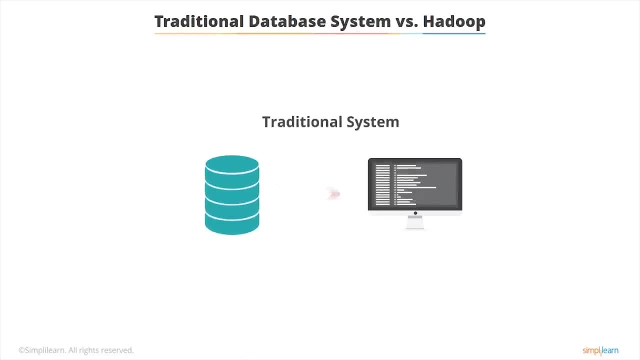 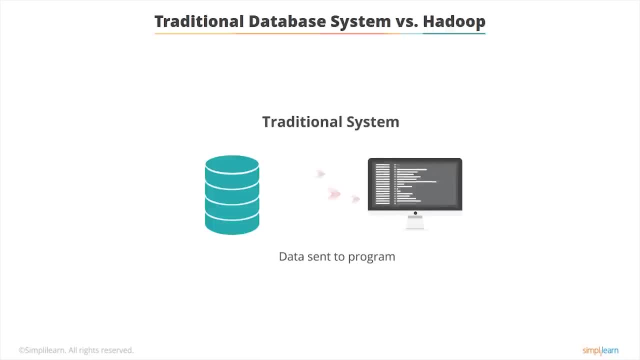 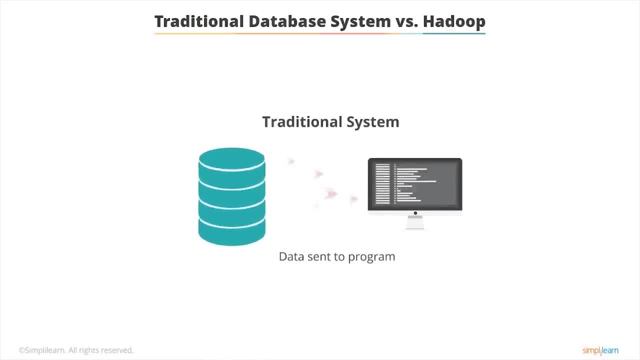 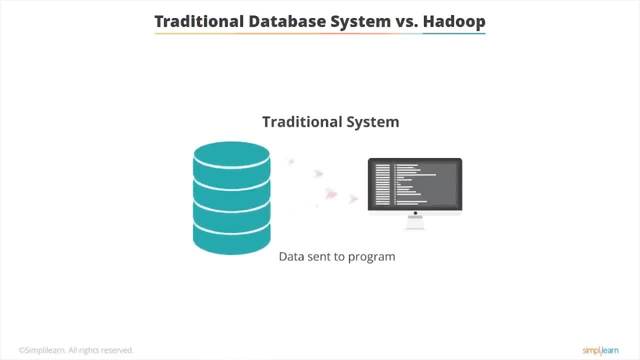 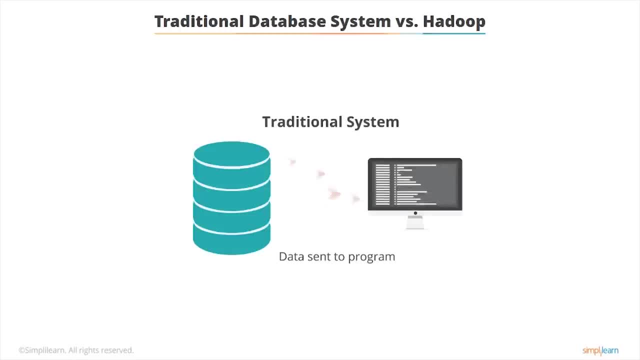 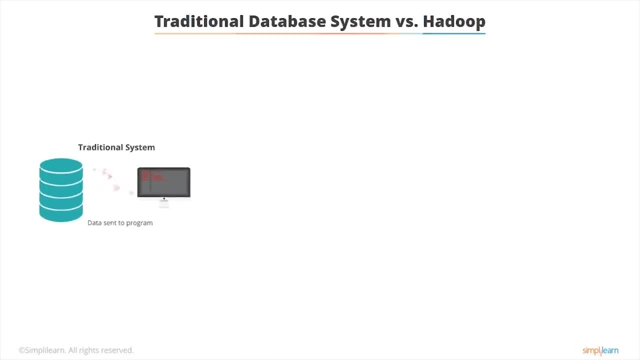 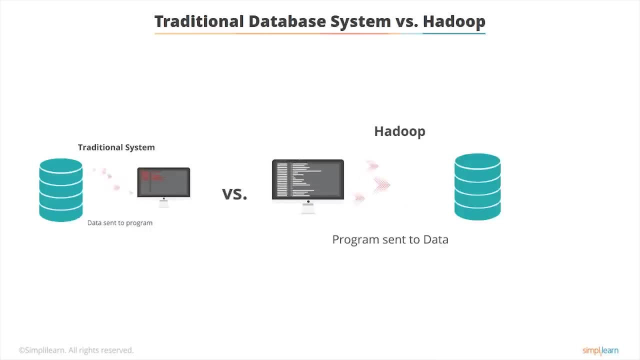 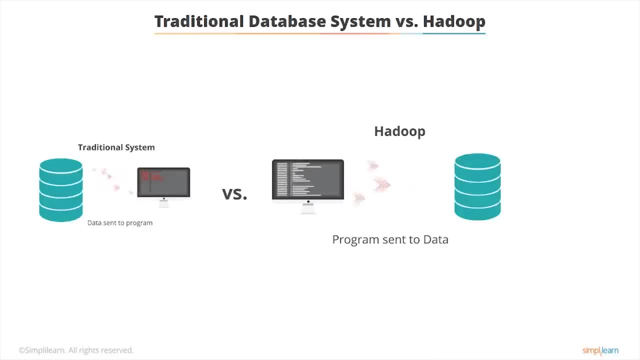 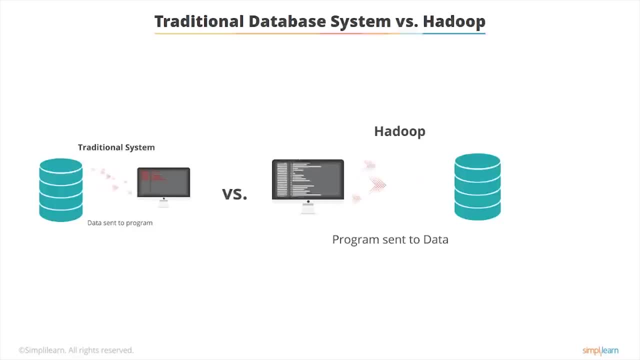 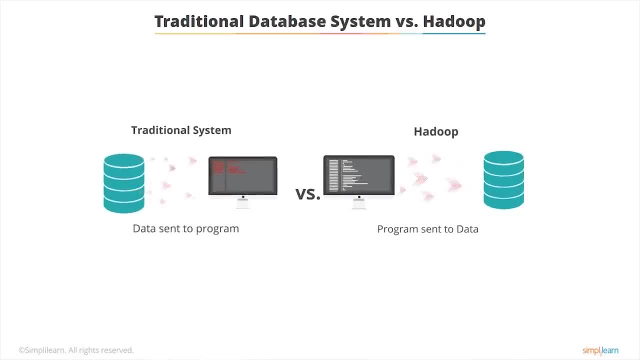 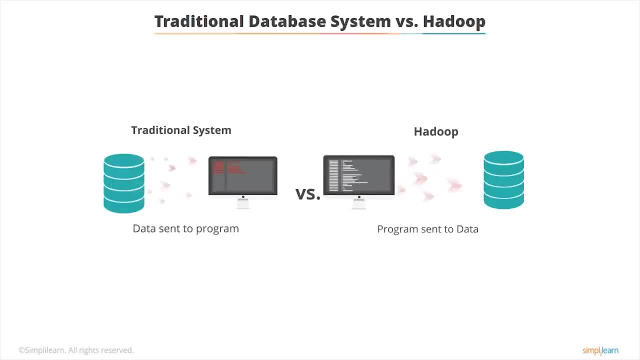 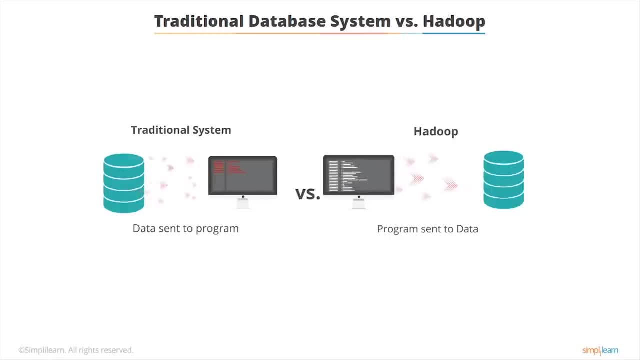 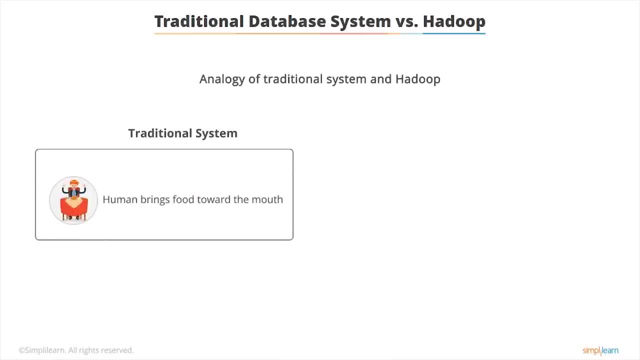 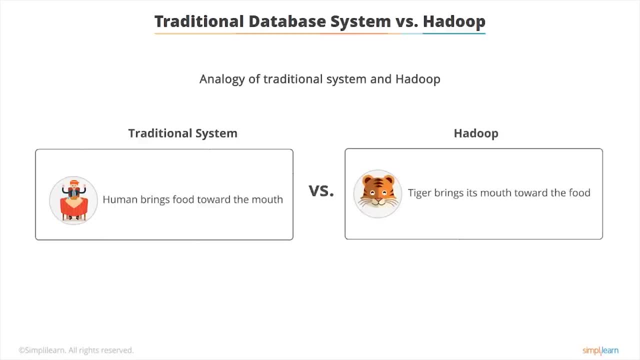 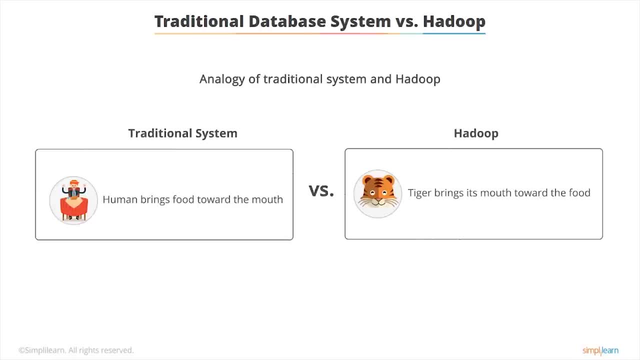 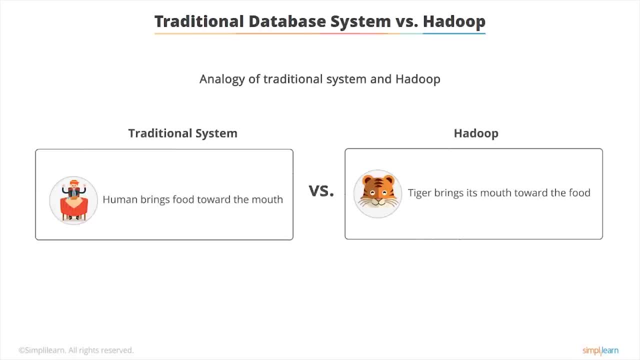 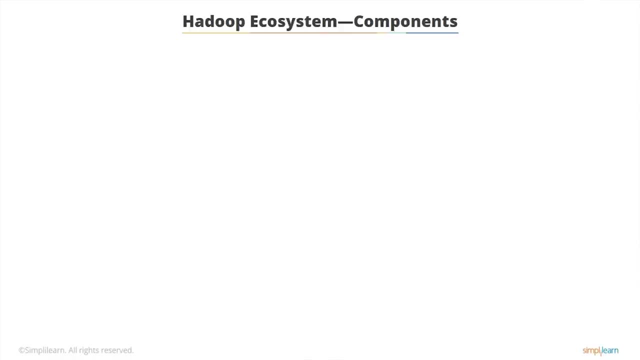 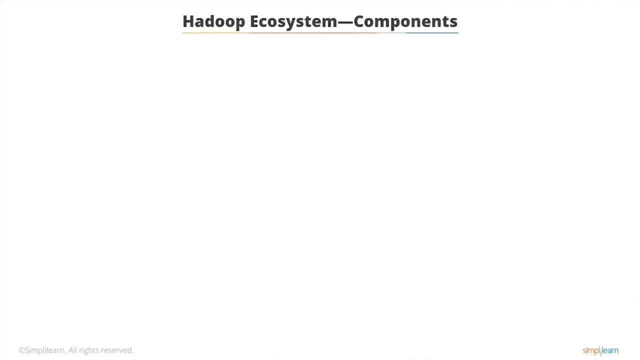 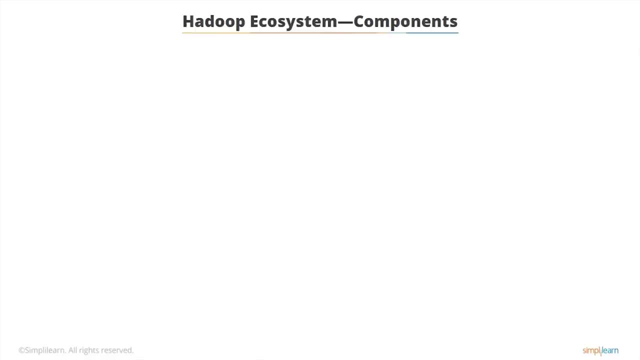 How does Hadoop solve the three challenges of the distributed system? you will learn the components of the Hadoop ecosystem and how they perform their roles during big data processing. The Hadoop ecosystem is continuously growing to meet the needs of big data. Let's understand the role of each component of the Hadoop ecosystem. 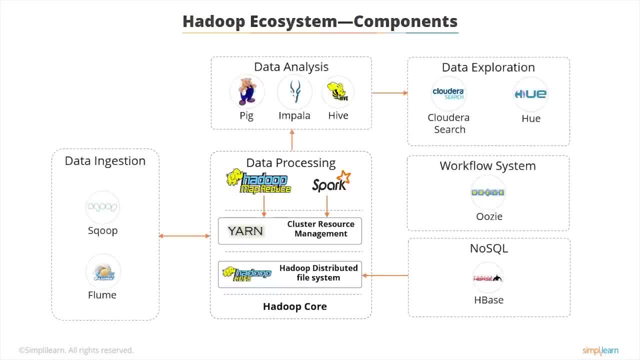 It's comprised of the following 12 components: Hadoop Distributed File System, HBase, Scoop, Flume, Spark, Hadoop, MapReduce, Pig, Impala, Hive, Cloudera's Search, Uzi, Hue. You will learn about the role of each component of the Hadoop ecosystem in the next screens. 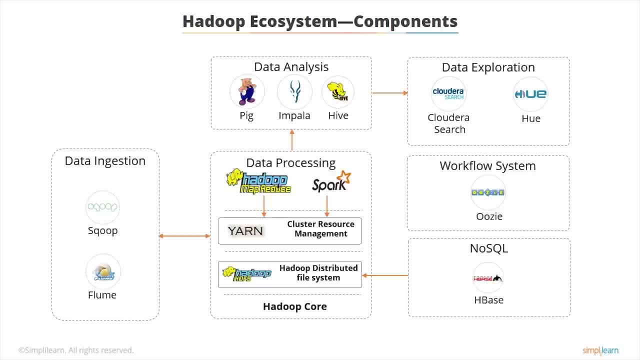 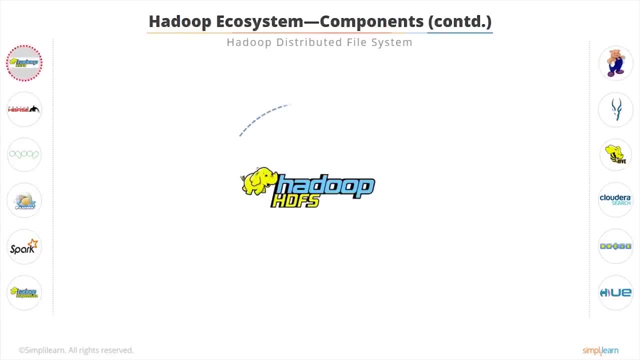 However, you will learn about YARN and its architecture in the next lesson. only Hadoop: Distributed File System. Let's understand the meaning and importance of HDFS. HDFS is A storage layer for Hadoop Suitable for distribution, Distributed Storage and Processing. That is, while the data is being stored, it first gets distributed and then it is processed. 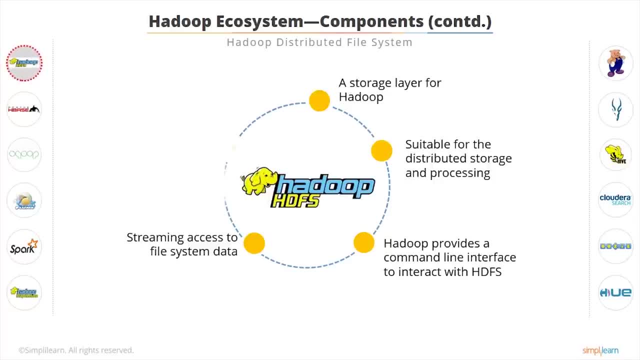 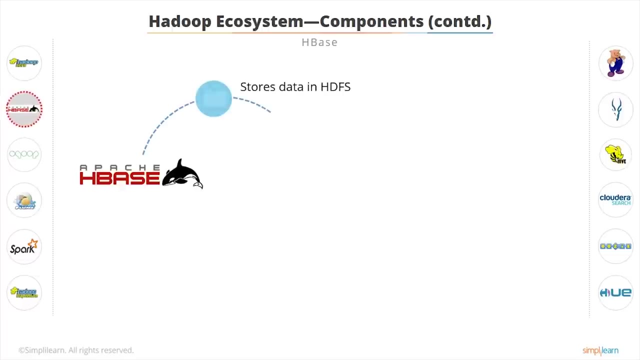 HDFS provides Streaming access to file system data, File permission and authentication. HDFS uses a command-line interface to interact with Hadoop. So what stores data in HDFS? It is the HBase which stores data in HDFS. HBase is a NoSQL database. 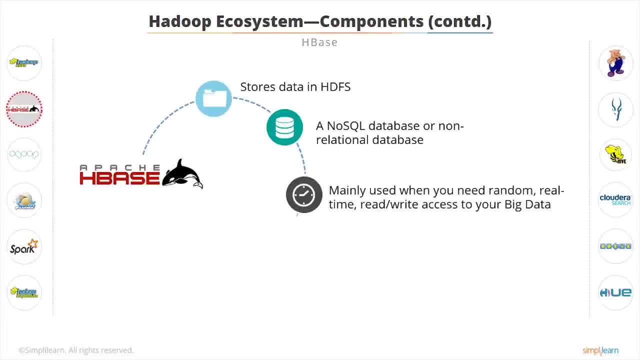 HBase is important and mainly used when you need random real-time read-or-write access to your big data. It provides support to high volume of data and high throughput. In an HBase, a table can have thousands of columns. We discussed how data is distributed and stored. 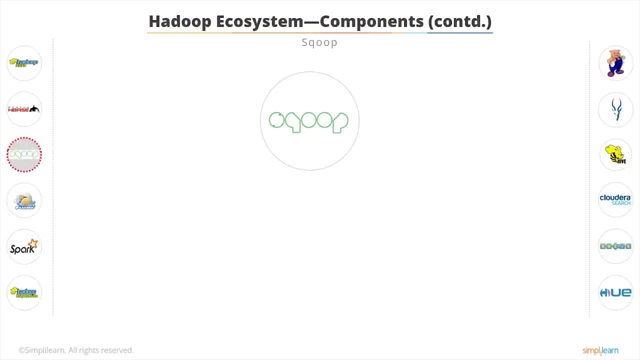 Now let's understand how this data is ingested or transferred to HDFS. It is done by Scoop. Scoop is a database. Scoop is a tool designed to transfer data between Hadoop and relational database servers. It is used to import data from relational databases such as Oracle and MySQL to HDFS. 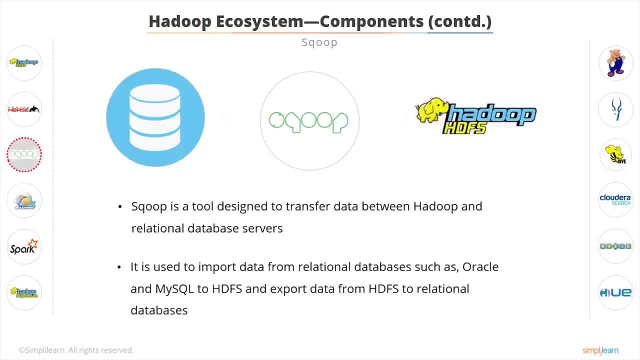 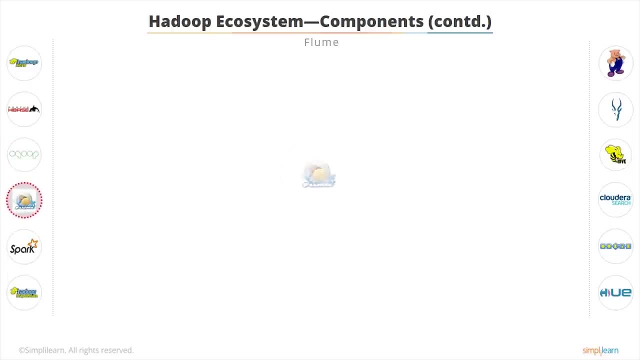 and export data from HDFS to relational databases. If you want to ingest event data, such as streaming data, sensor data or log files, then you can use Flume. Flume is a distributed service that collects event data and transfers it to HDFS. 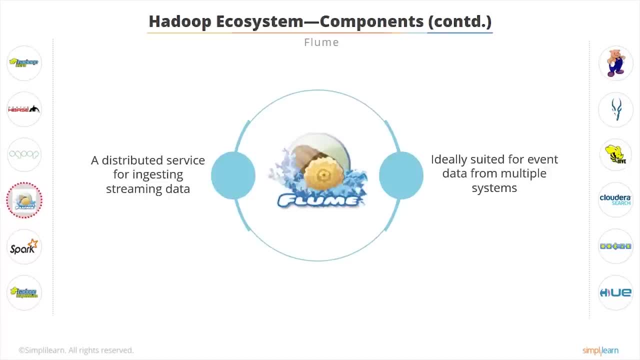 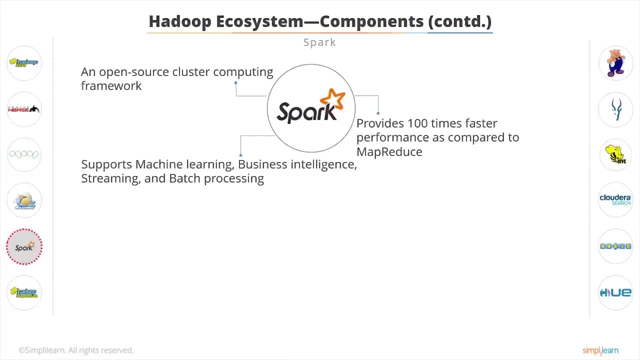 It is ideally suited for event data for HBase. After the data is transferred in the HDFS, it is processed. One of the framework that processes data is Spark. Spark is an open-source cluster computing framework. It provides up to 100 times faster performance for a few applications with in-memory primitives. 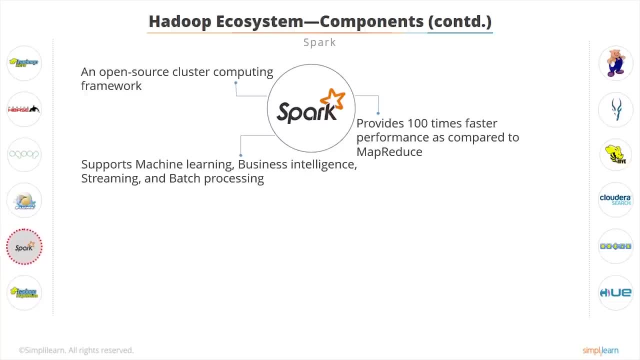 as compared to the two-stage disk-based MapReduce paradigm of Hadoop. Spark can run in the Hadoop cluster and processes data in HDFS. It also supports a wide variety of workload, which includes machine learning, business intelligence, streaming and batch processing. 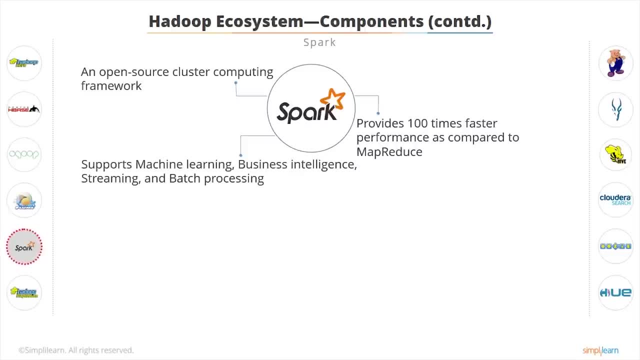 Spark has the following major components, as shown in the diagram: Spark Core and Resilient Distributed Datasets, or RDD, Spark, SQL, Spark Streaming, Machine Learning Library, or NLIB, and Graphics. Spark is now widely used and you will learn more about it in subsequent lessons. 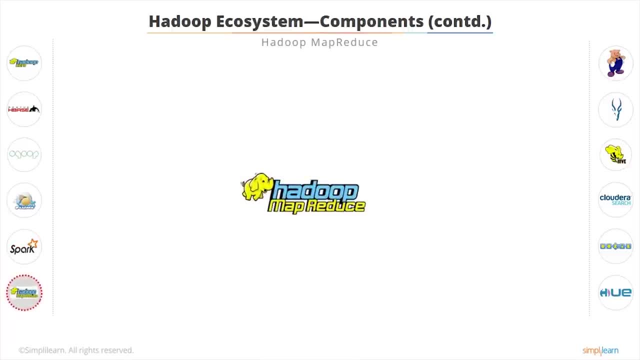 Hadoop MapReduce is the other framework that processes data. It is the original Hadoop processing engine, which is primarily Java-based. It is based on the Map and Reduce programming model. Many tools, such as Hive and Pig, are built on MapReduce model. 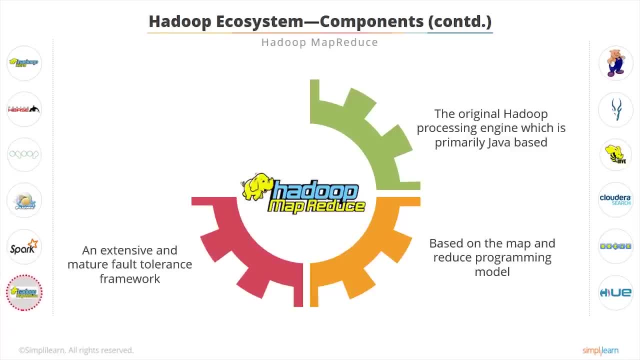 It has an extensive and mature fault tolerance built into the framework. It is still very commonly used but is losing ground to Spark. After the data is processed, it is analyzed. It can be done by an open-source high-level data flow system called Pig. 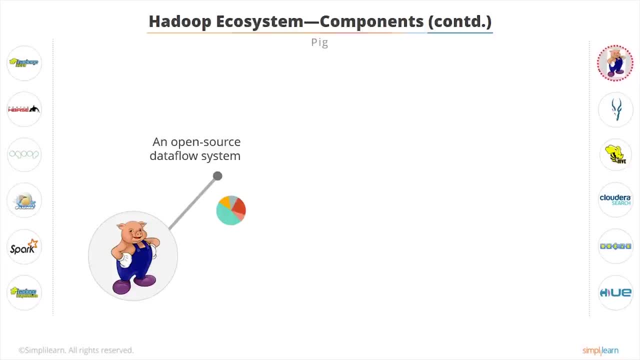 It is used mainly for analytics. Pig converts its scripts to Map and Reduce code, thus saving the user from writing complex MapReduce programs. Ad hoc queries like Filter and Join, which are difficult to perform in MapReduce, can be done easily using Pig. 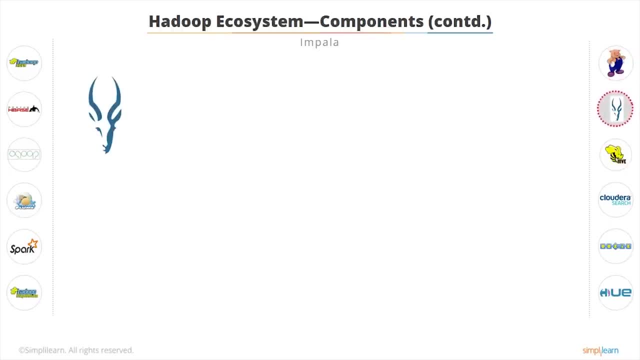 You can also use Impala to analyze data. It is an open-source, high-performance SQL engine which runs on the Hadoop cluster. It is ideal for interactive analysis and has very low latency, which can be measured in milliseconds. Impala supports a dialect of SQL, so data in HDFS is modeled as a database table. 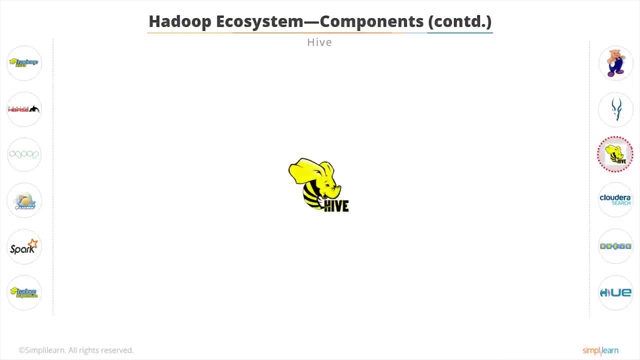 You can also perform data analysis using Hive. It is an abstraction layer on top of Hadoop. It is very similar to Impala, However it is a bit more complex. However, it is preferred for data processing and extract-transform-load, also known as ETL operations. 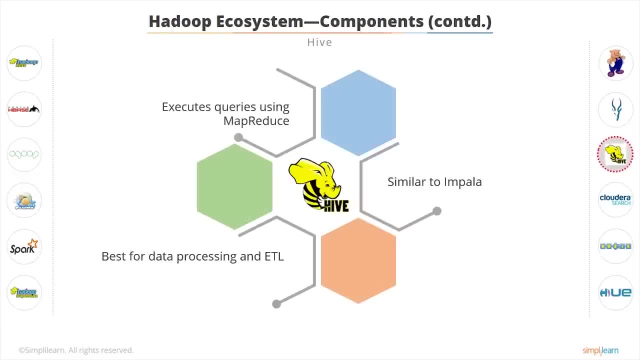 Impala is preferred for ad hoc queries. Hive executes queries using MapReduce. However, a user need not write any code in low-level MapReduce. Hive is suitable for structured data. After the data is analyzed, it is ready for the users to access it. 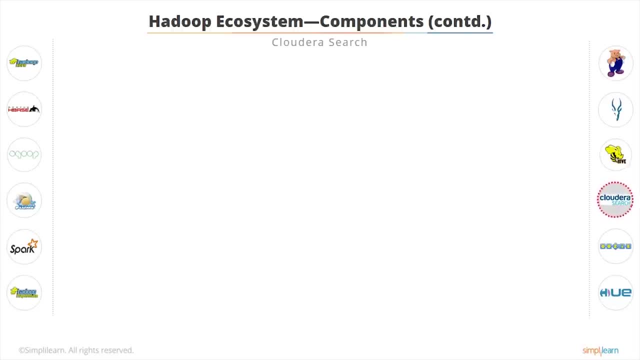 What supports the search of data? It can be done using Cloud Era's Search. Search is one of Cloud Era's near-real-time access products. It enables non-technical users to search and explore data stored in or ingested into Hadoop and HBase. 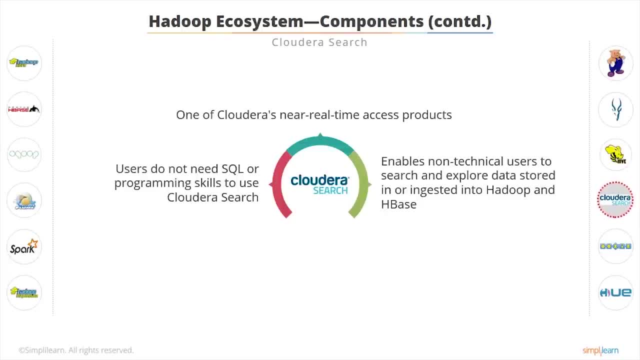 Users do not need SQL or programming skills to use Cloud Era's Search, because it provides a simple full-text interface for searching. Another benefit of Cloud Era's Search, compared to standalone search solutions, is the fully-integrated data-processing platform. Cloud Era's Search uses the flexible, scalable and robust storage system included with CDH or Cloud Era's distribution, including Hadoop. 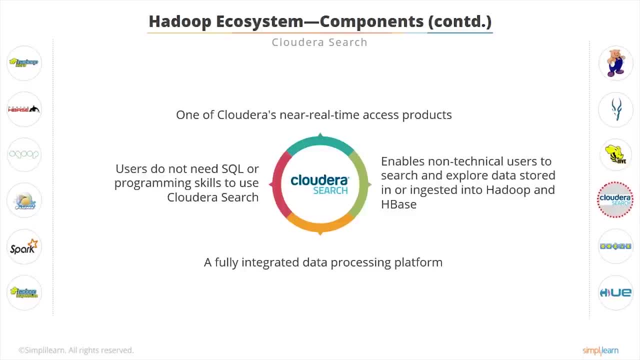 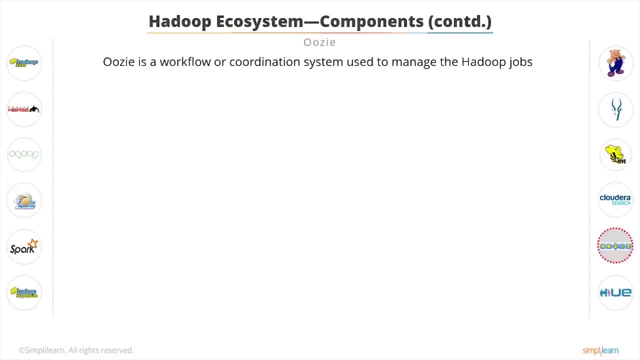 This eliminates the need to move large datasets across infrastructures to address business tasks. Hadoop jobs such as MapReduce, Pig Hive and Scoop have workflows. Uzi is a workflow or coordination system that you can use to manage the Hadoop job. 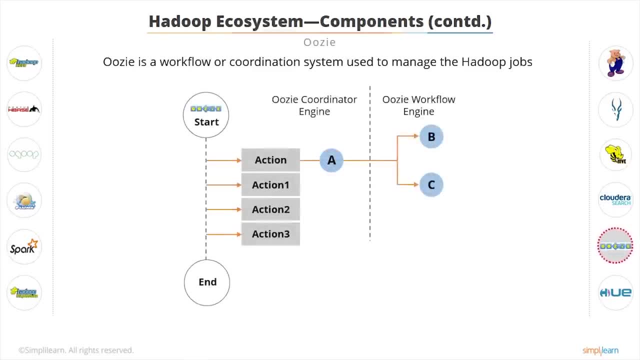 Uzi application lifecycle is shown in the diagram. As you can see, multiple actions occur between the start and end of the workflow. Another component in Hadoop ecosystem is HUE. HUE is an acronym for Hadoop User Experience. It is an open-source web interface for Hadoop. 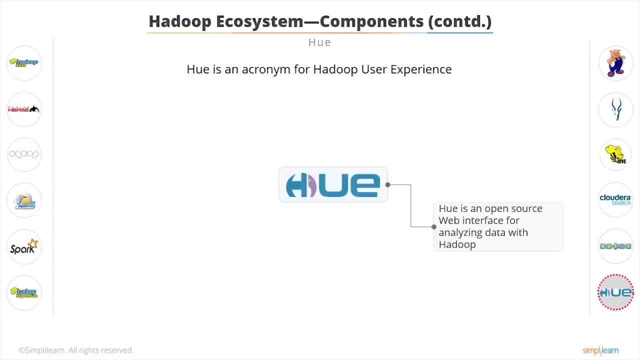 You can perform the following operations using HUE: Upload and browse data, Query a table in Hive and Impala Run, Spark and Pig jobs and workflows. Search data. HUE makes Hadoop easier to use. It also provides SQL editor for Hive, Impala, MySQL, Oracle, PostgreSQL, SparkSQL and SolarSQL. 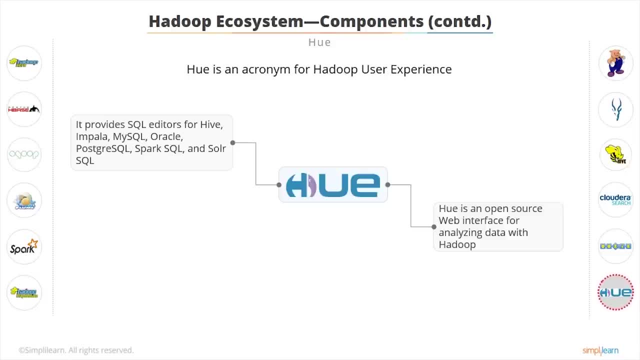 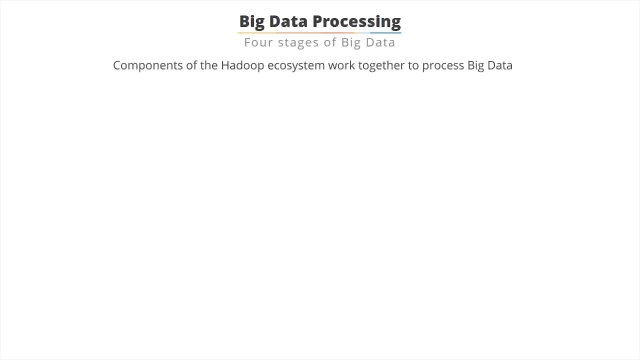 We will learn more about HUE in our future lessons. After a brief overview of the 12 components of the Hadoop ecosystem, we will now discuss how these components work together to process big data. There are four stages of big data processing: ingest- 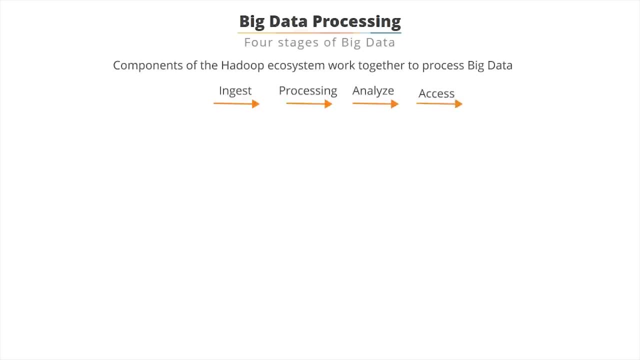 processing, analyze access. The first stage of big data processing is ingest. The data is ingested or transferred to Hadoop from various sources, such as relational databases systems or local files, As discussed earlier in this lesson. you know that Scoop transfers data from RDBMS to HDFS. 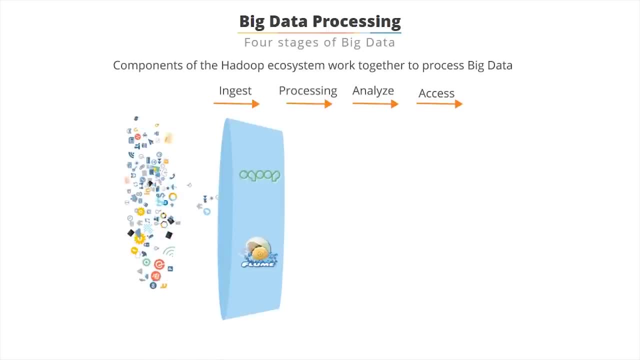 whereas Flume transfers event data, The second stage is processing. In this stage the data is stored and processed. We discussed earlier that the data is stored in the distributed file system HDFS and the NoSQL distributed data HBase. 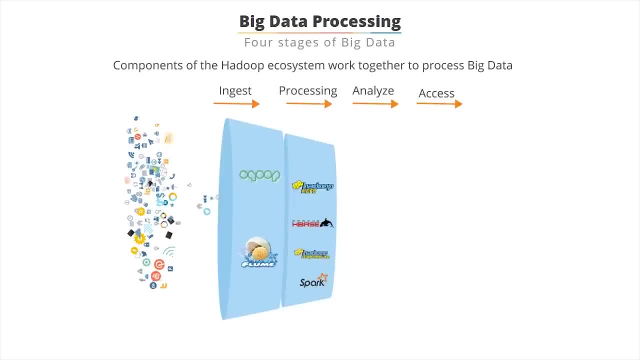 Spark and MapReduce perform the data processing. The third stage is analyze. Here the data is analyzed by processing frameworks such as Pig, Hive and Impala. Pig converts the data using Map and Reduce and then analyzes it. Hive is also based on Map and Reduce programming.